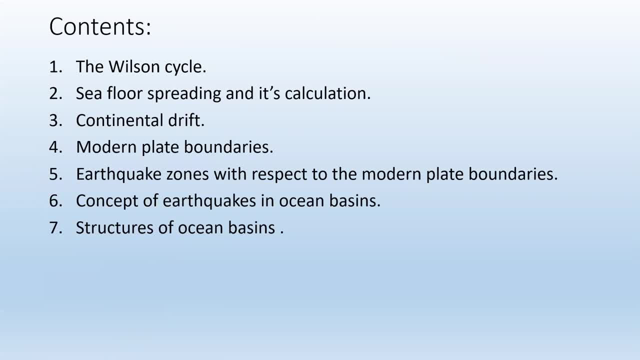 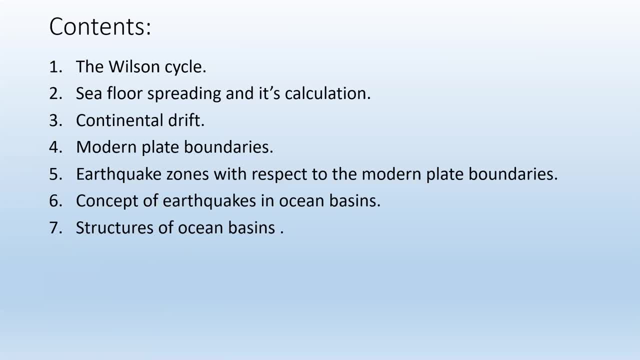 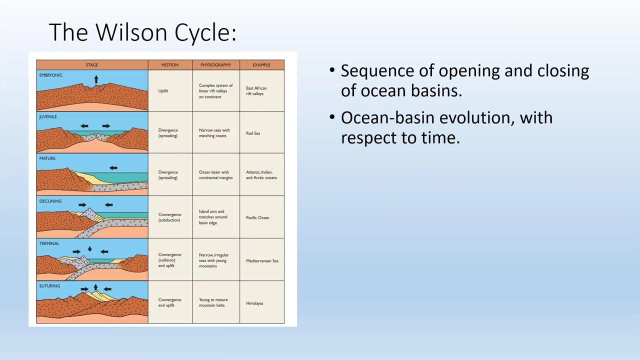 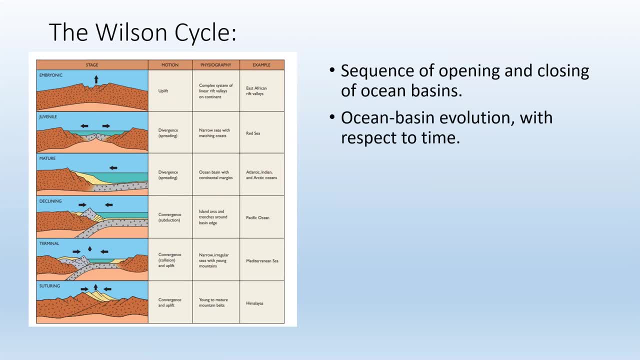 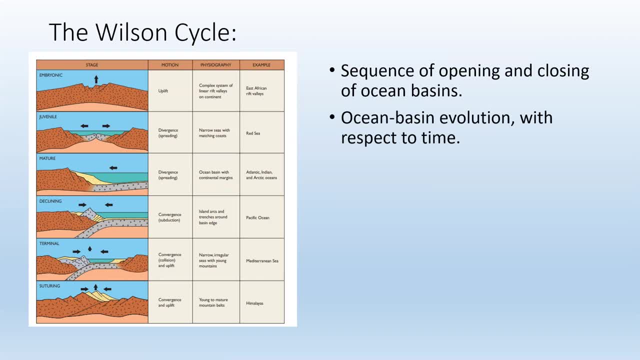 and closing of ocean basins and the ocean basins evolution with respect to time. this can say you. uh, now you can see that arabali mountain belt. it is very highly mineralized deposits that um the world. let's think deposit. all those things are there, but think about those things, those are. 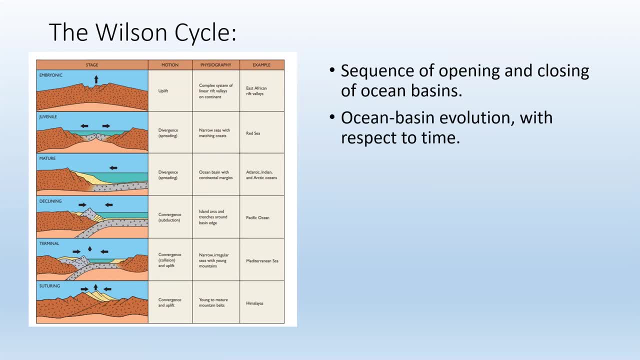 once upon a time those are a part of ocean basins. now those are very beautiful hilly mountains. so how these types of things develop, how those opening and closing of ocean basins occurs, all these things the wilson cycle can describe you here. in the first diagram you can see that 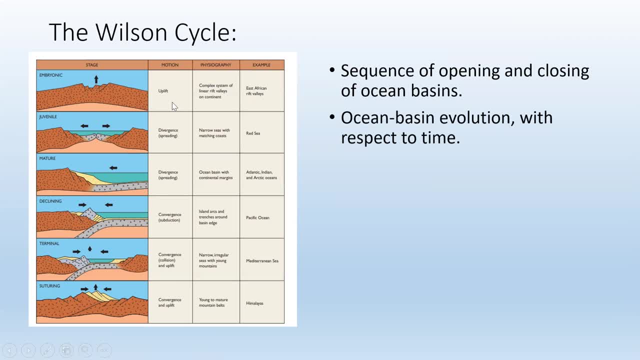 there is a uplift, uplift in motion and the complex system of linear rip valleys on continents. here, because of upliftment, there is a tension developed and because of the tension, two sides of the plates, two sides of the plates move apart and because of this, one juvenile ocean, juvenile basin forms. 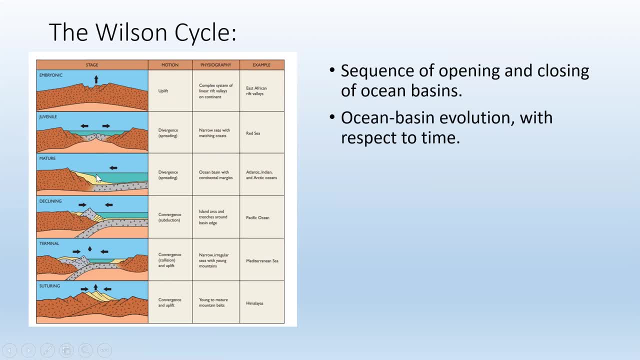 then, because of this diver, juvenile basin, juvenile basin forms and you can see these types of divergence in modern sea, in modern area, modern time, in red sea, red sea is growing. right now there is a tension and because of the tension, red sea is growing day by day. okay and uh stay, uh, with mature stage, there is diverging and spreading. 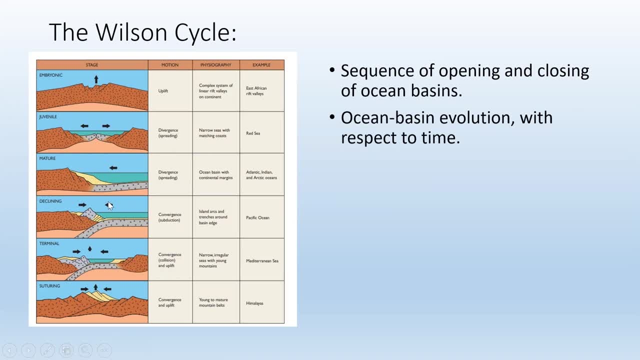 uh of these plates occurs and uh after that at the. at the end they, though those plates, collide with the continental plates or or another oceanic plates. in the subduction zone where a christianity plism develops- and because of this there is upliftment- develops. in the subduction zone where a christianity plism develops, and because of this there is upliftment. 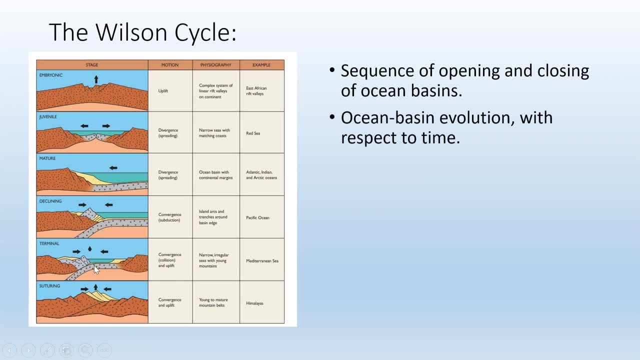 develops in the subduction zone, where a christianity plism develops and because of this there is upliftment trends, are the products of these types of subduction areas. and finally, the ocean basin close in the convergent boundary. so this is the sequence of wilson cycle. in the next slide we will discuss about the 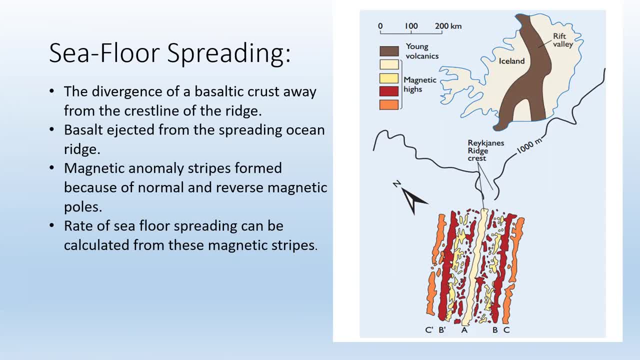 sea floor, spreading all those things that is the sea sea is generating in the mid-oceanic ridges, where the hot molten magma comes in the surface of the ocean and from there the ocean basins, develops the divergence of a basaltic crust away from the crest line on this ridge, that means in the mid-oceanic ridge. 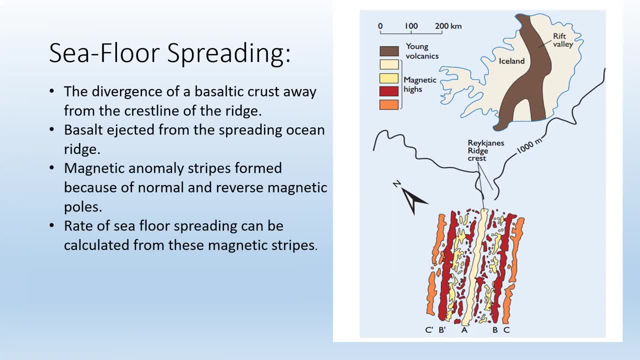 where there is divergence, that is, that means the two plates move apart from each other, new hot molten magma comes, and this molten magma forms the new basaltic crust on the ocean surface. the next difference is that the scale reacts to the human surface of the ocean. 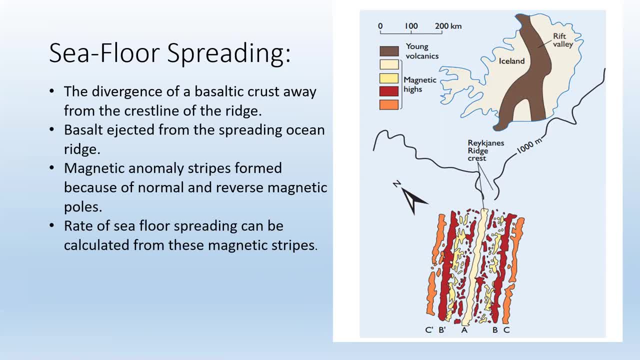 there are many groups that also joke that on the ocean surface we have massive 很 v Ар curvอ and that is because of enormous energy and the atmosphere in ocean surface. texts on that basically means the Beatitudin islands has an activityart番. 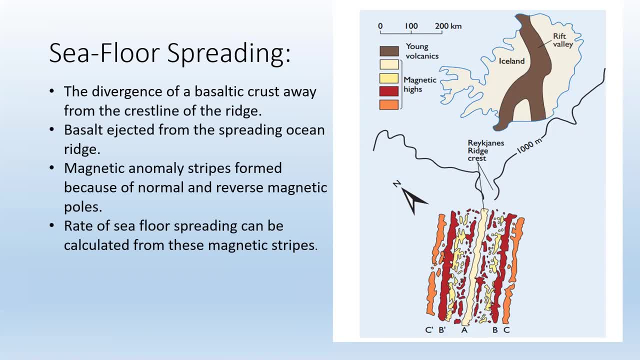 vaan, It becomes a Maya medium external. so accordingly different magnetic stripes forms and with the help of these magnetic stripes in in both of the parts of that mid-oceanic ridge we can calculate the rate of sea floor spreading from these magnetic stripes. here in this diagram you can see that this is a ridge crest and these 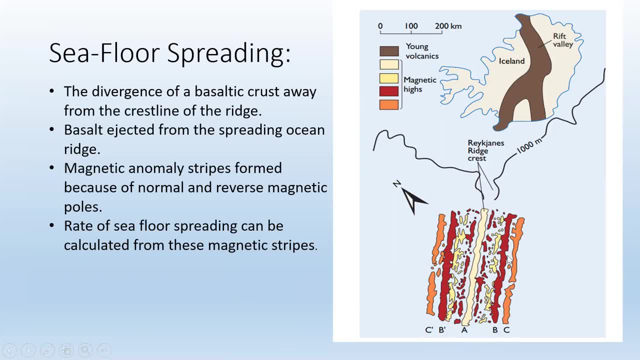 are b, b dash, c, c dust. these are the different magnetic stripes. look c and c does. they are once formed together. they were once in the position of a. now they are apart from each other and they are recording their, their paleo pole position and everything. so this is the. 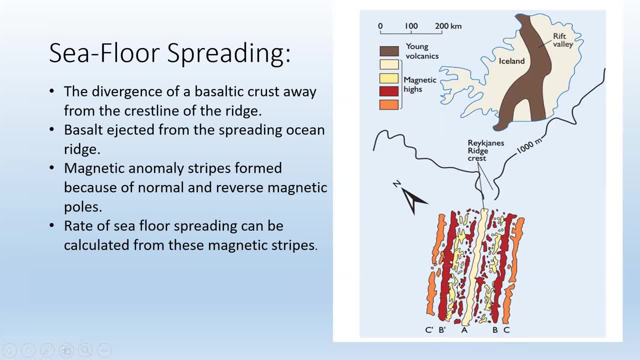 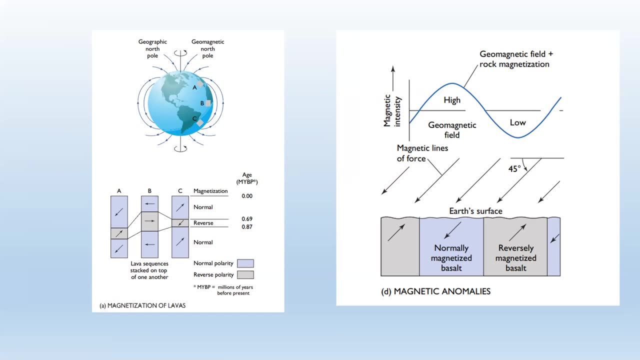 form of now the magnetic and normal and reverse magnetic poles. and now we can go to the next slide where we can easily here you can easily understand that how these normal and reverse magnetic poles formed. look at the. this image here is geographic north pole and this is. 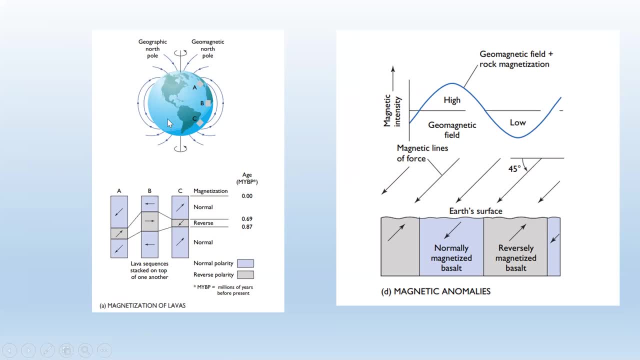 the south pole, and this is the geomagnetic north pole. geomagnetic south pole is also there. so when the magma erupts it takes the thermal remnant, magnetization of that geomagnetic pole, that thermal remnant. when the magma get cooled they take the present position of that geomagnetic pole. 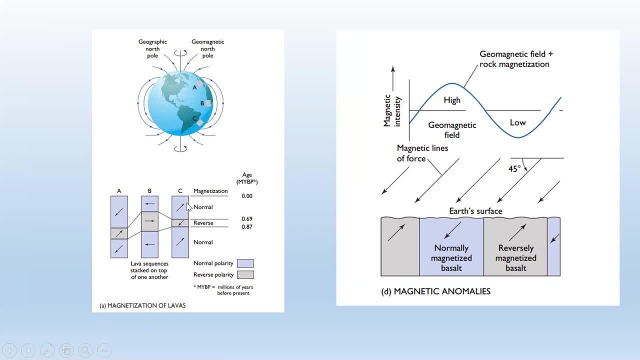 here you can see that there are normal and reverse. normal and reverse magnetization with respect to edge. when the magma erupt they were in the normal magnetic poles. they were, they were parallel to the normal magnetic poles. and then, with respect to time when another magma eruption takes place, the geomagnetic pole was reversed. so it records. 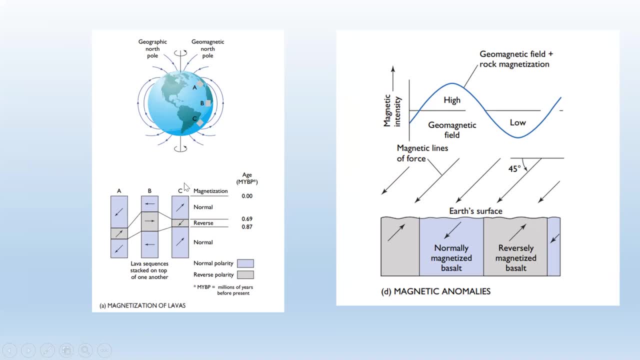 the then time of magnetic pole position. then again it takes the position of normal magnetic poles with respect to the geomagnetic field of the earth. so all these normal reverse magnetization stripes represent the present magnetic pole of that time when that magma erupted, when that magma cooled, and they take 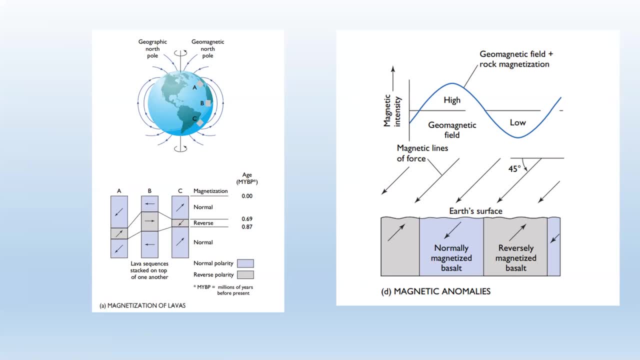 the thermal remnant magnetization of that time and they represent the geomagnetic pole position of that time. so this is the magnetization of labhas in this diagram we are showing. now think about how we can understand that these magnetic anomalies, this is normal, reverse, normal, reverse. 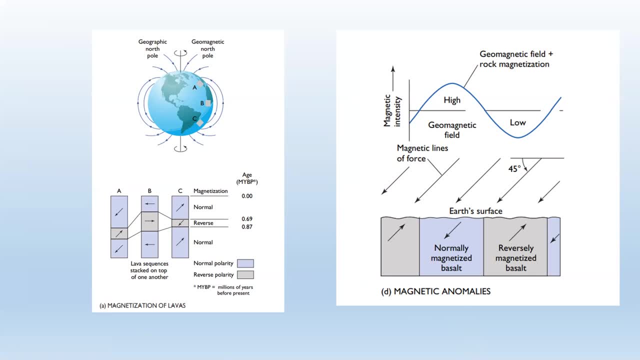 how think about the present magnetic position? okay, when it is now normally magnet, normally magnetized. so when we go to the field and we take the magnetic intensity values, now it is normal magnetized field. when we find any normal magnetized basalt, it will add with the present 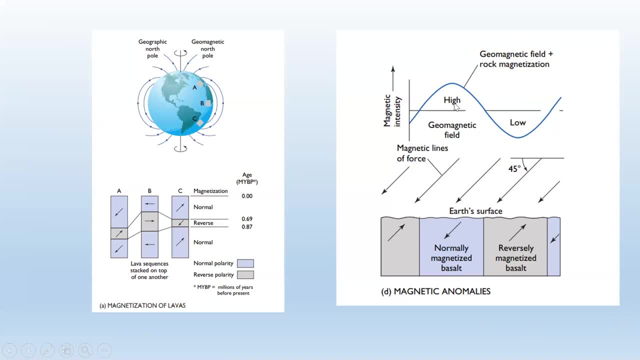 value. so it will give the high, high magnetic intensity. but when we will find any reverse magnetized basalt- because the present magnetic field is normal and we are finding something reverse- it will give you some negative value. look at this, that negative value add plus and plus will. 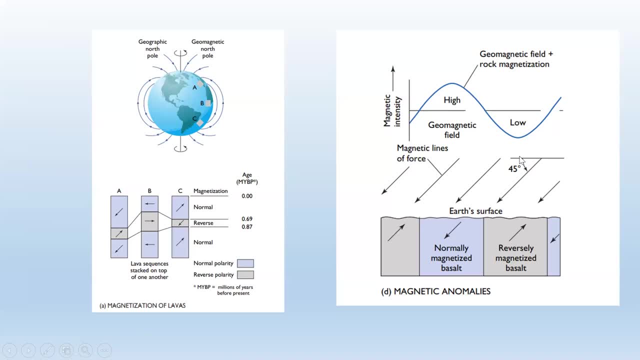 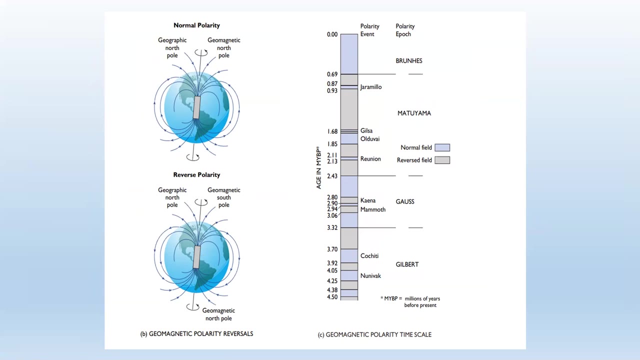 give you add, but plus with minus will give you something low. so here this: magnetic anomalies we can easily found in field with the magnetic intensity detectors. now in the next slide we will go to some important magnetic polarity time scales. think this: magnetic polarity time scales are very 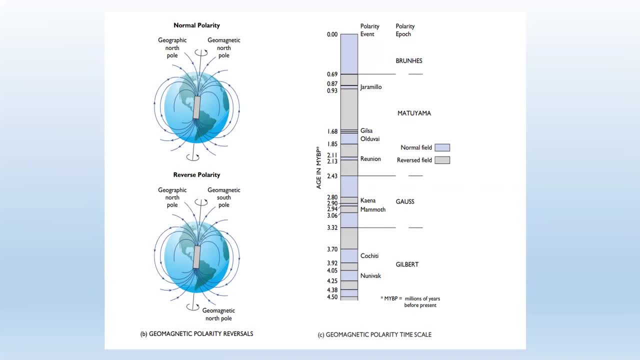 important not only for these are only coming in exams or some csr net exams, but also for these are very important for oceanographic researches. you can see that, gilbert goss, machuama, brunes, these are the polarity epochs and here, with respect to time, 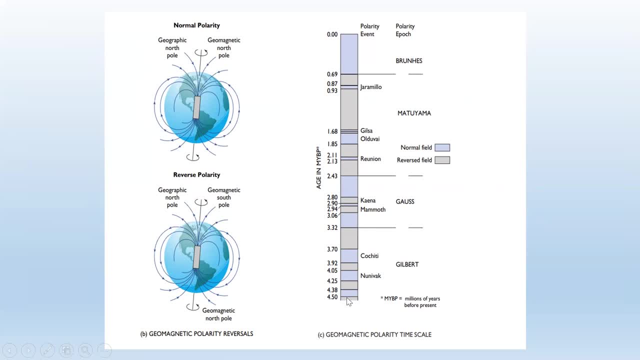 can see that how they are representing the normal and reverse magnetic field with the earth: normal polarity stripes and reverse polarity stripes. now, geomagnetic north pole is here and geomagnetic north pole is also here, so these are the normal polarity here. geographic north pole is here, but 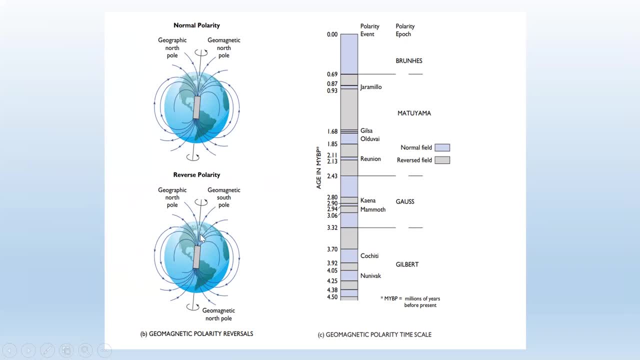 geomagnetic south pole is here, it just get reverse. so this is the reverse polarity. how this normal and reverse polarity happens? it is because the convection currents of the outer core and the mantle, the inner core, is solid, when inner, inner, and it can rotate and because of this a geodynamic, geodynamic formed and that 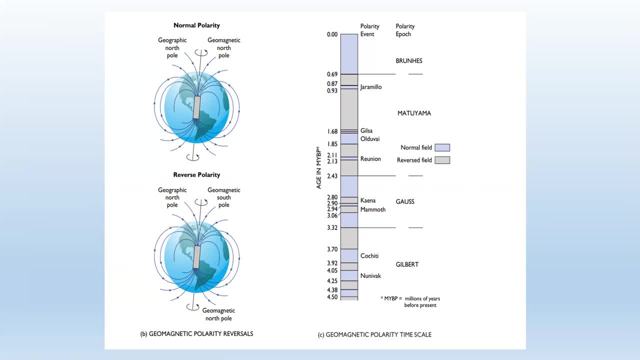 gives you the magnetic position of the earth, so from there we can get the magnetization effects of the earth. so now in this picture you can easily understand when the geomagnetic pole and the geographic not pole is, or like is, superimposed one upon another or they. 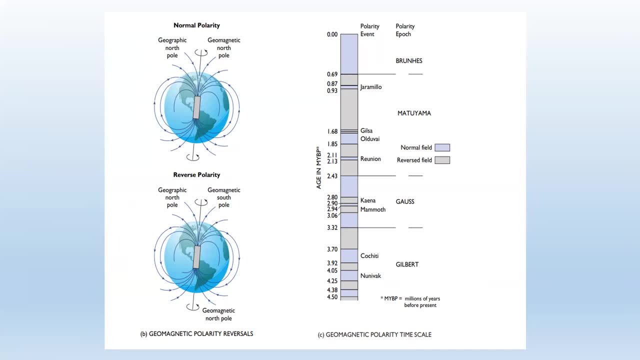 are just in one direction, that we can say as normal polarity. but when they are just rivers, that means your graphic, not pole, comes with the geomagnetic south pole, we can say it a reverse polarity, and all those things are happening. one of the reason is the geodynamic 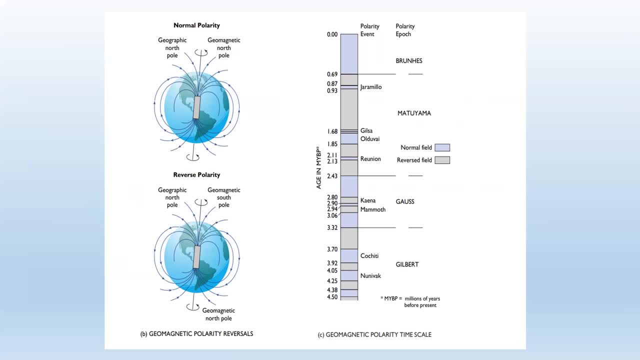 effect of the earth and the movement of the inner core, solid inner core which is composed of nickel and iron, with that a hot molten outer core. so, because of this normal and reverse polarity, different geomagnetic polarity forms with respect to time. these are gilbert goss, matriama and brunus. 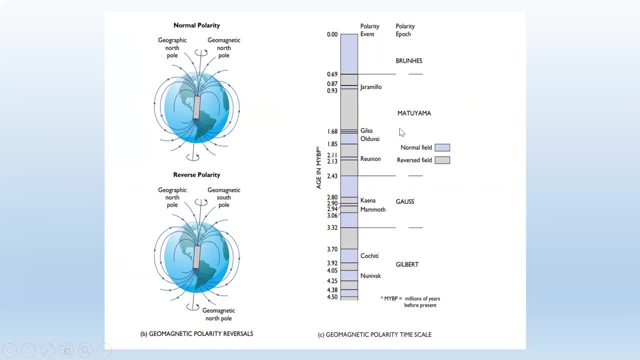 with respect to age, if you see that the matriama is mostly reverse in field. some also positive or normal is there, but mostly it is reverse. but look at brunus, it is the mostly in normal field, so that pole position changing is recorded with this geomagnetic polarity time scales. 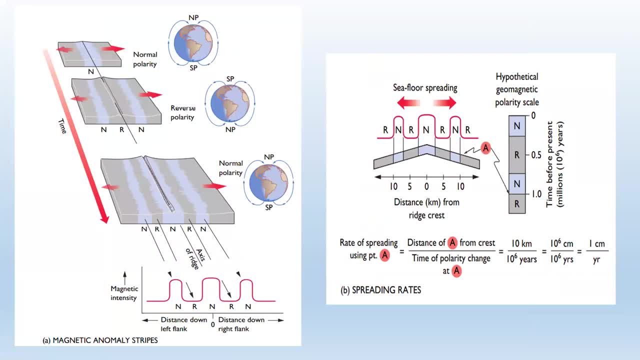 now, in the next slide we will see how to calculate the spread in rates with these geomagnetic a pole positions and the distance from their polarity change from the kick crest of that mid oceanic reach. here you can see that this is the normal and reverse- normal and reverse position of those mid oceanic range or ocean reach, basalt stripes, and this is 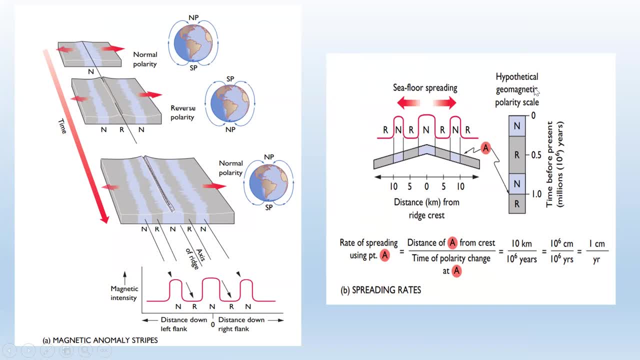 thus this is showing the sea floor spreading and this is the hypothetical geomagnetic polarity scale. now take it: reverse normal, reverse normal. now here is a point a: how we can calculate the rate of spreading of that position a from the mid oceanic reach. they are moving apart from each other, but we know that they are moving from apart. 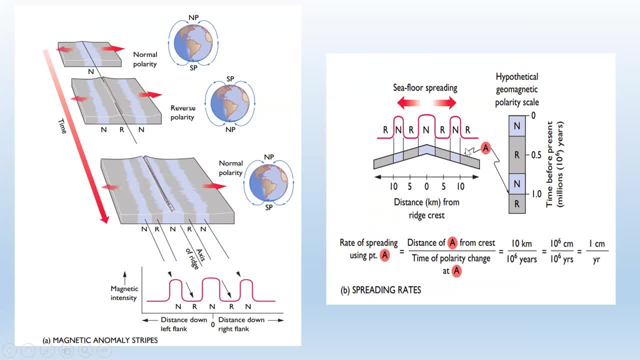 from each other, but how to calculate the rate. so for the, for this calculation, we have to know the a from the crest, from this is the crest, and we have to know that distance, simply so, here it is 10 kilometer. then the time of polarity change: it is 10 to. 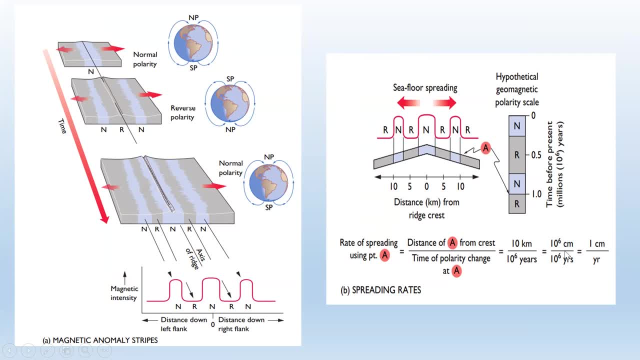 the power 6 years here. so now we can say that it is 1 centimeter per year of that position. of rate of spreading at the point a. similarly we can also correlate. we can also take until the rate of spreading of any points if you rate of. 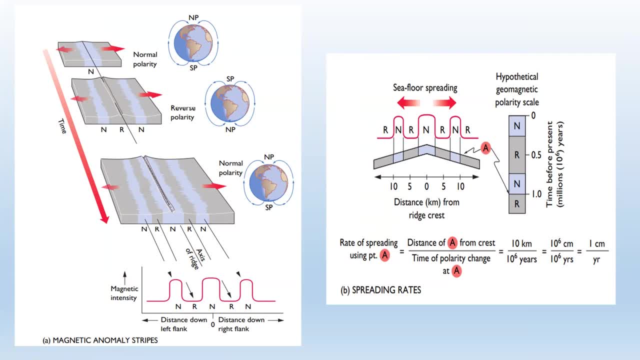 spreading of any point. if you see the art map, the plates and the motion of those plates are not the same everywhere. somewhere it is to millimeter from your. that is not Atlantic. somewhere it is 160 millimeter per year, that is is specific rise, somewhere it is. 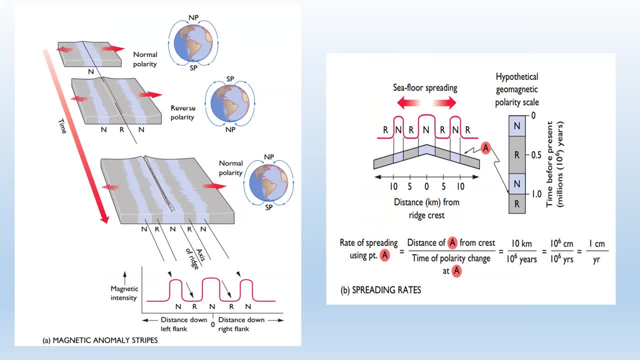 10 millimeter per year between Africa and Eurasia. here the closer of basins occurs somewhere. it is 80 millimeter per year. that is between Nazca plate and South America plate. the last two is the model gives the rates of closer, closer, and the first two is the separation of the motion. so you can see that the rate. 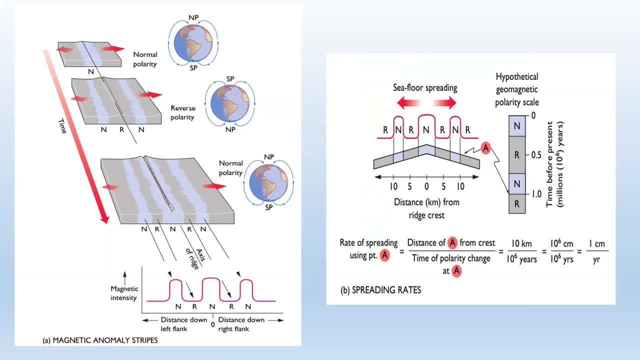 of motion is not everywhere the same, so it is very necessary to calculate the rate of spreading. so to calculate it, this formula, we can directly use it here. we can use the distance a from the crest and then time of polarity change, and that at that point these are showing the magnetic anomaly stripes of along the 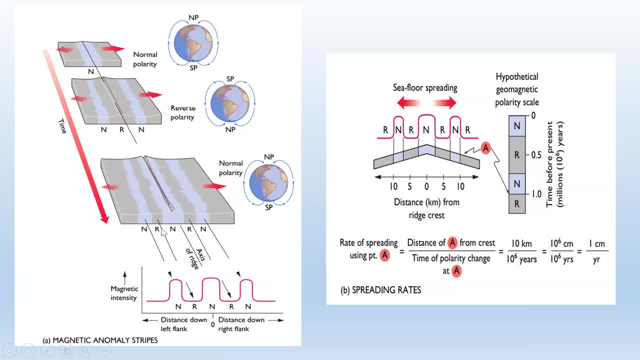 mid-oceanic ridges. this is the. this is the mid-oceanic ridge and along the divergent motion, the magnetic anomaly stripes are false with respect to the present, with respect to the present position of magnetic pole of that time. so this is simple to calculate. 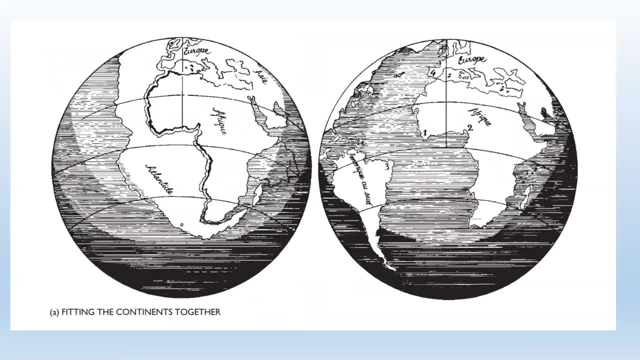 the rate of spreading at any point. now we will go to the continental drift. now we are going to say about continental drift. if you see the present world map, you can see. If you see the present position of India, America and different plates of South Africa, Australia, you can see that there is a zigzag, puzzle type of structure. 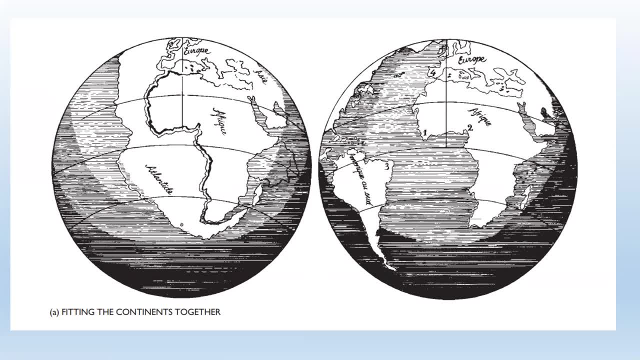 The African plate and the South American plate are a part of a zigzag puzzle, and the Indian plate and the Australian plate are also another part of zigzag puzzle. So what these things indicate If you think about that continental drift, there are some evidences that this drifting of those continents occurs. 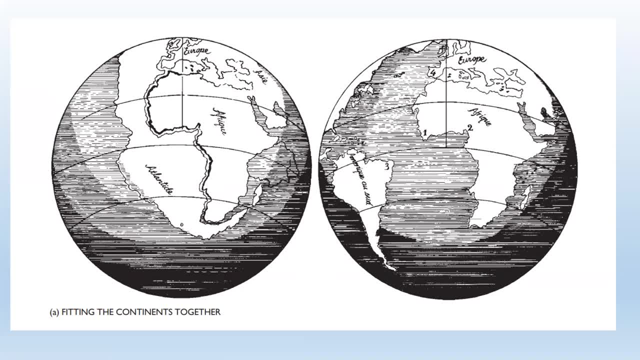 That is the parbo carboniferous glaciation. Think about the glacial evidences of Talchir, that is in the lower Gondwana, Below the Rannigans, Colberts and Nassau. This Talchir glaciation event is found in so many places. That is, in Africa also, in Australia also. 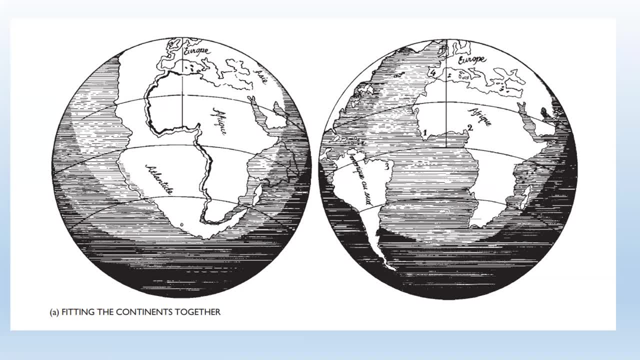 Maybe the name is different, but the time span and that glaciation events, they are recorded in different continental parts. So this is the evidence, This is one big evidence that that continental drift happens. And then again it comes: the Gondwana Colberts. 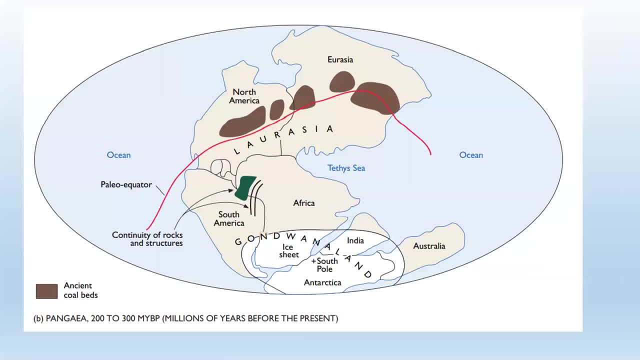 The Gondwana Colberts. The Gondwana Colberts are found in different parts in Africa, South America also, and Australia, India, all those places the same Gondwana Coalfield is found. In India these Gondwana Coalfields are found along the Damoda Valley, along the Mohanadi Valley, some important coal bearing horizons, at the Rannigan, Jharia, Jharia, etc. 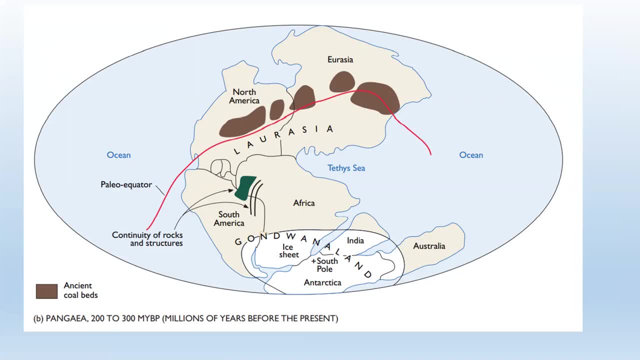 Jharia is giving us coal from last 100 years or more than that. So these are the very important, economically important places of India. Then there is another evidence that traces of opposite continental margins. Look at the South American plate and the African plate. 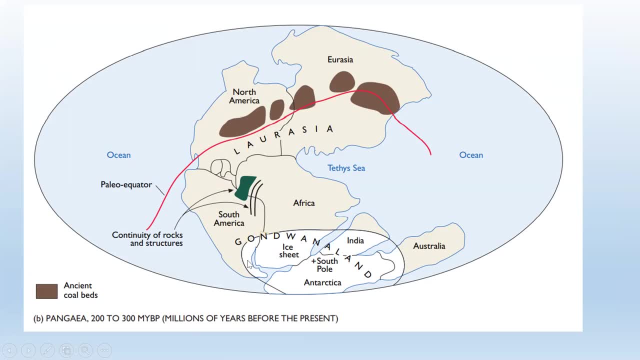 And if you I told you that there was a zigzag puzzle like structures- Indian plate, Australian plate- If we take all the continental Plates together, there is a matching boundary. So this is the traces of opposite continental margins. So this indicates that once upon a time all these plates were together and then they moved apart. 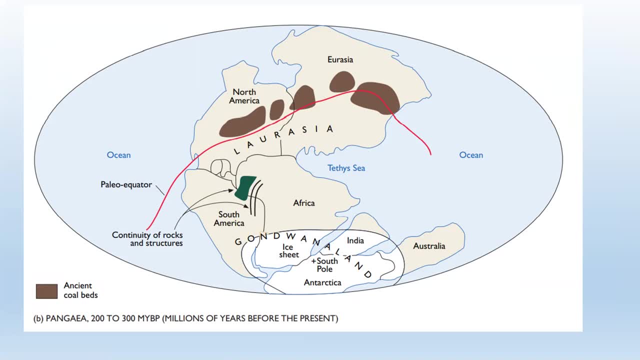 And now they are at their present position, They are not attached with each other, But with that boundary we can say that once upon a time they were together. and again also, with their apparent polar wandering, But Of different positions, of that different plates, we can say that these, even these continents were once upon a time, were together. 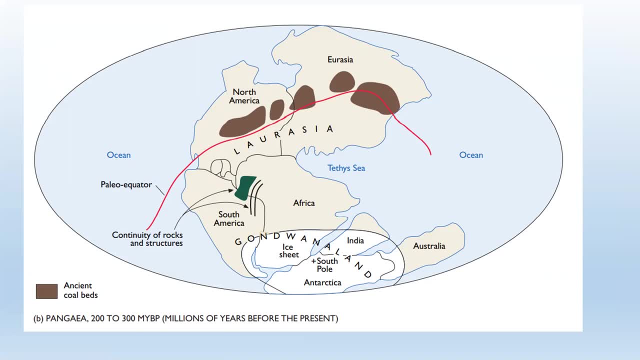 So these are the main evidence of continental drift, that is, permacarponiferous glaciation, Gondwana coal beds, traces of opposite continental margins, apparent polar wandering. But other than this, so many evidences are there like that Gondwana flora. 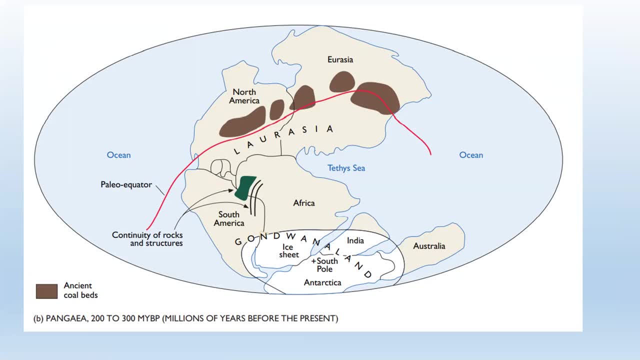 That is, glossopteris gangomopteryx, and all those lower Gondwana flora you can find in South Africa also, you can find in Australia also, along with India. So these are the so many evidences are there of those continental drifts, one by one. 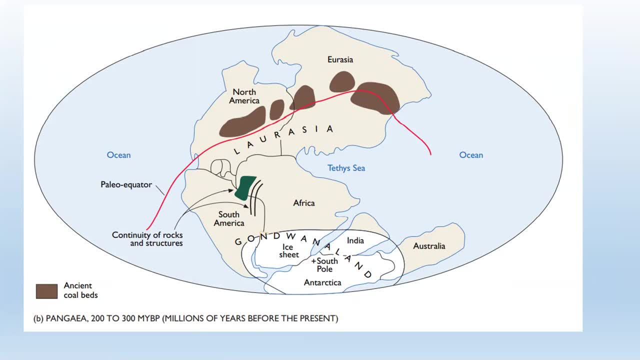 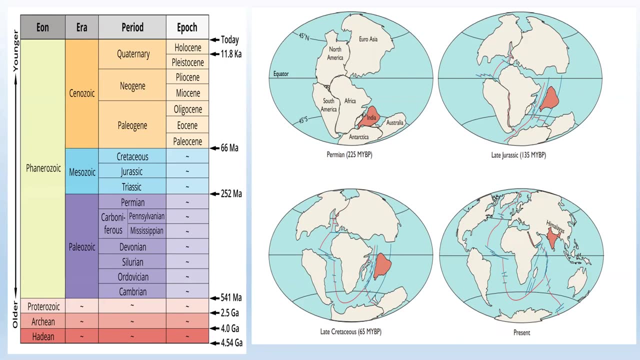 But now we will focus on the continental drift and we will move apart that how many times this continental drift occurs with respect to geological time. So if you take this geological time scale, so many times There are these continental drifts happens in the Cambrian. Gondwana land very likely existed as a supercontinent, coexisted with three other cratonic centers. 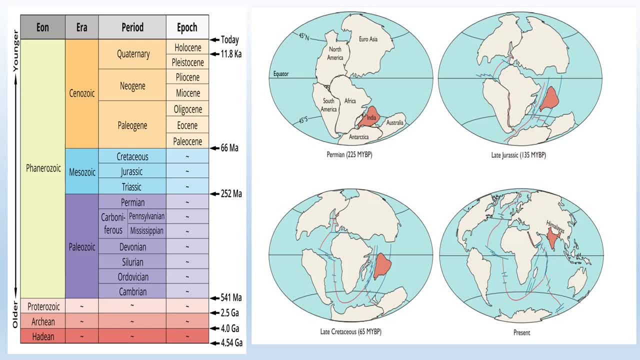 Laurasia, Baltica and Siberia. Laurasia is nothing but North America and Greenland, and Baltica is Northern Europe and Siberia. in the Cambrian they were together and after that they moved apart. then in the Silurian, Laurasia and Baltica. 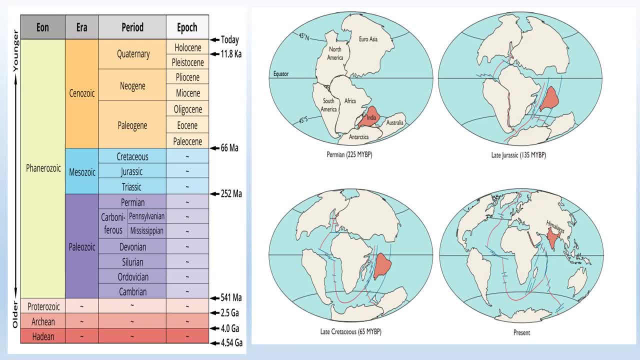 Then in the Silurian, Laurasia and Baltica Fused together during the Caledonian Orogeny and the gap between lower Gondwana and Laurasia closed. at Silurian Devonian boundary and the Silurian Devonian boundary the gap between Gondwana and Laurasia closed. that is in the 410 million year and this is called the Acadian Orogeny, and in the late Devonian Laurasia separated from Gondwana land. 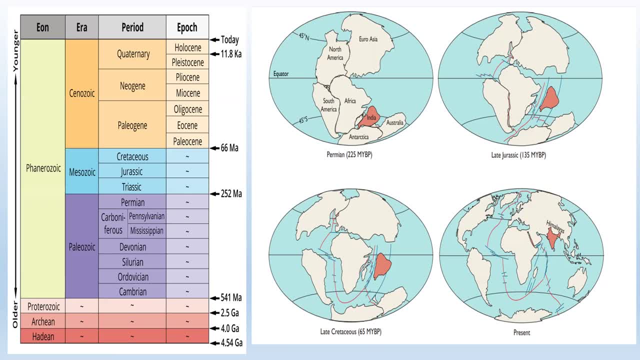 Fused together during the Caledonian Orogeny and the gap between lower Gondwana and Laurasia closed. that is in the 410 million year and this is called the Acadian Orogeny, and in the 410 million year Laurasia separated from Gondwana land. then in the late Carboniferous, that is, in the 350 million year, collide, the collide again in the during the Hyrcenean Orogeny. 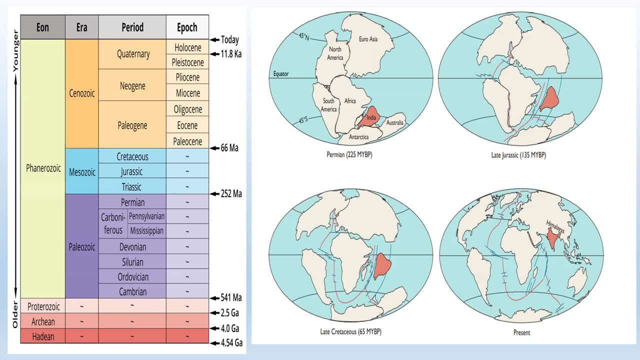 By the late Carboniferous Pangea was complete, that is, during the 300 million year. This is the very important time period, that is the late Carboniferous the Permian, That is, that is, the late Carboniferous the Pangea was complete and after that, during the Permian-Jurassic. 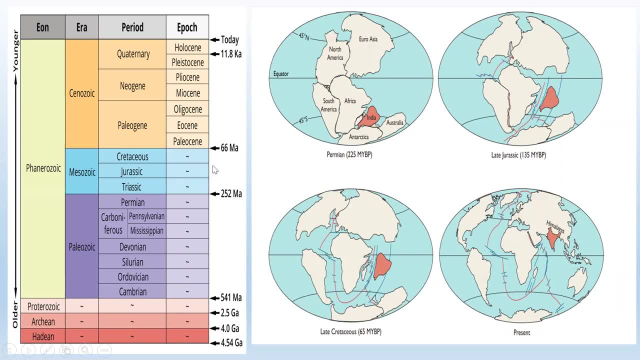 time the Pangea was together. Pangea existed in late Paleozoic and early Mesozoic. Their dispersal into their present position took place largely in the late Cretaceous and Tertiary. So you can see the evidences of those different types of fossils and different types of coal beds. 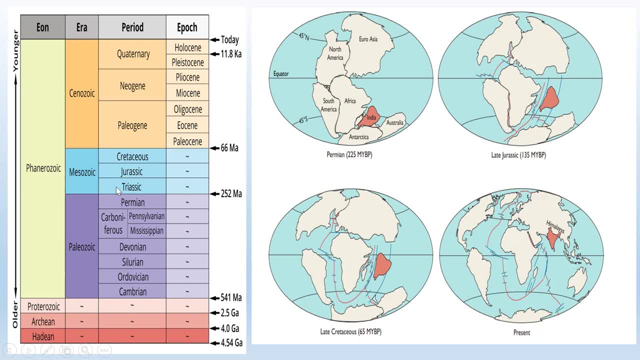 different types of lower Gondwana fossils and some Jurassic, that is, the Lystrosaurus fossils of Runnigan area and all those things you can see in those, these Pangea in different parts of Gondwana land, because Pangea was existed during the late Paleozoic and early Mesozoic times. 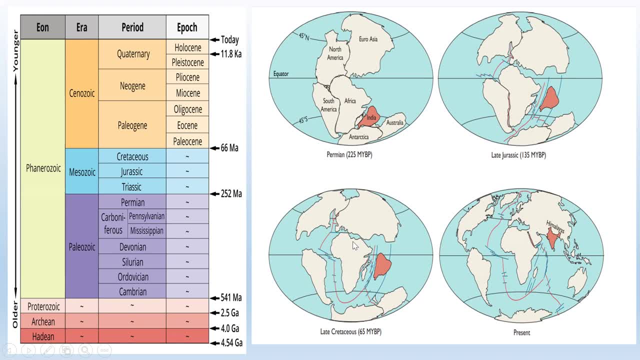 Then in the late Cretaceous, there was another late Cretaceous. you can see in this that is the 65 million year when the Deccan volcanic events also started. they moved apart and they started their migration from their Gondwana position and now at the present, this is the world map and here all the continents were once. 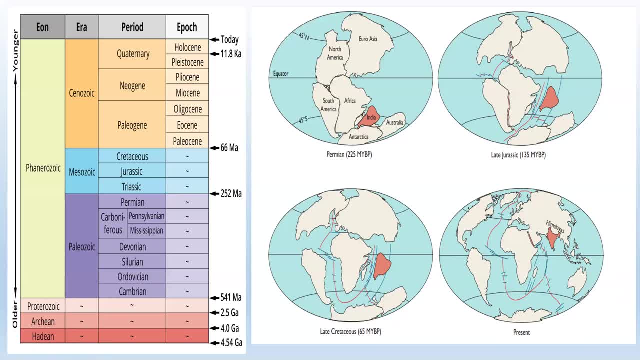 all the continents. they are the that they once upon a time, those which were in a southern continent, we can see now in the northern hemisphere. not all, but mostly they are. they comes in the northern hemisphere, they took a northward journey and this is the present position of all those continents. 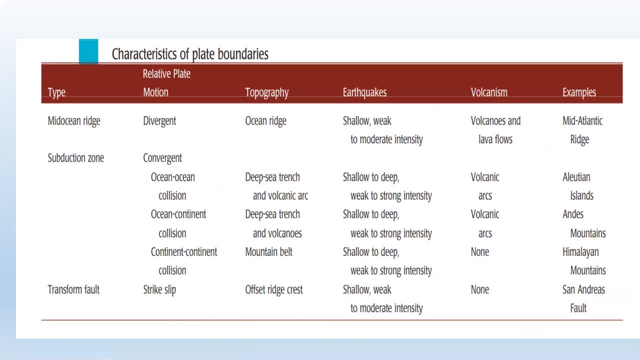 at present time. now, if on here we in the last place we share about the continental drift, and now you should know about the some pro modern examples of those different types of boundaries, that is, the mid oceanic reach subduction zone, that is the transcom poles. there are some. this table will show you some modern examples, that is. 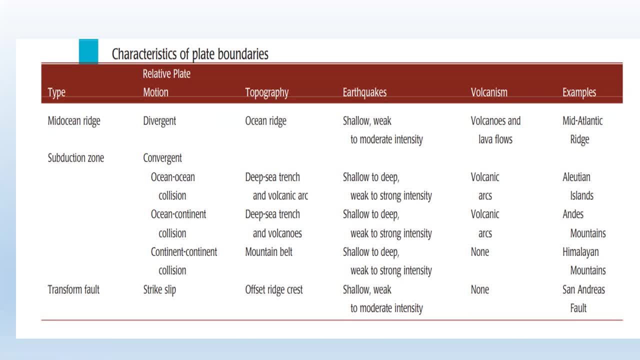 mid-atlantic reach. mid-atlantic reach, it is the, I think mid-atlantic is the modern ocean and so means mid-atlantic Atlantic is growing now it is the modern ocean, so mid-atlantic reach is a very beautiful example of mid-oceanic reach. 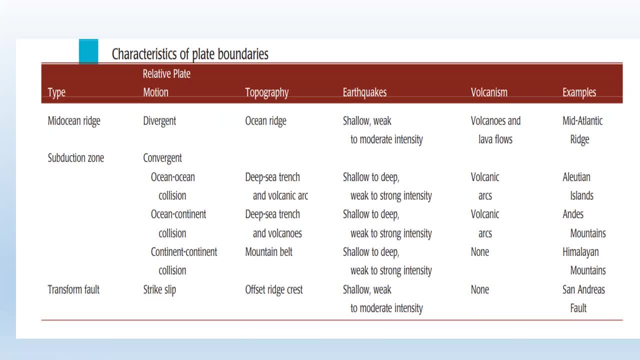 here divergent of plate occurs if you go to the subduction zone, the Aleutian Islands, and these mountains, Himalayan mountains, all those mountain chains, they are the subduction zones. here in the Himalayan mountains, continent, continent collision occurs, that is, the Indian plate collide with Asian plates once. 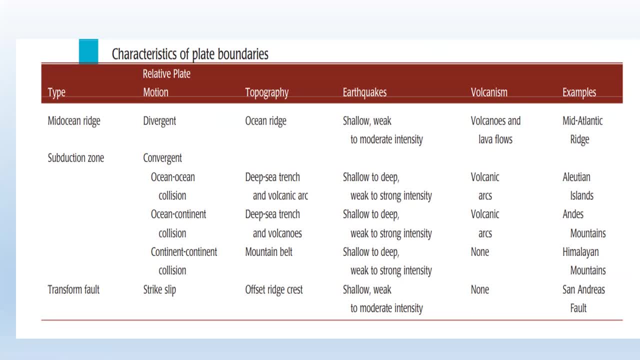 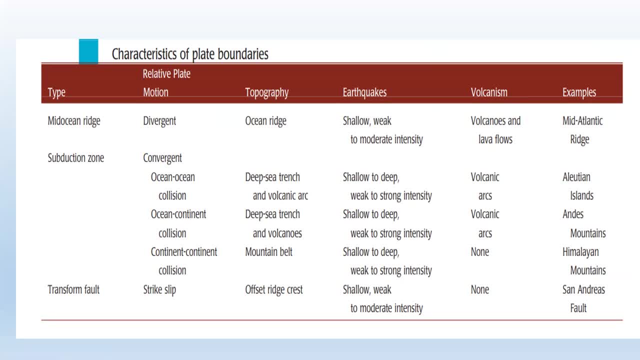 are also present in there, that Himalayan mountain belts, these. these are the evidences of those tethys sea and the basaltic events of those, the basaltic events of those. see, all those things are very beautifully present on those ophiolite complexes and the San Andreas fault is an example. 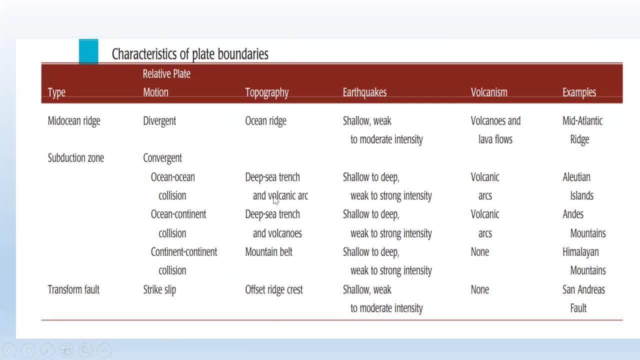 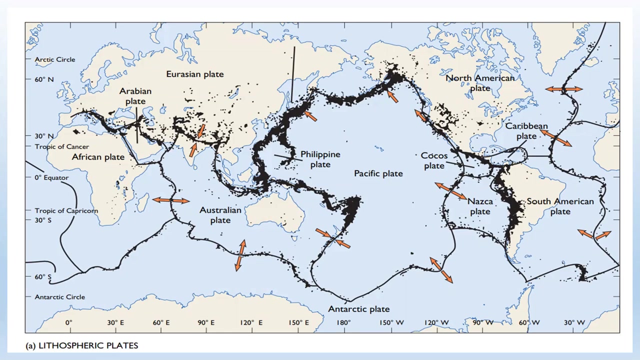 of transform fault in present date where there is very shallow to weak to moderate intensity earthquakes. these are the. these are these. these are the this table showing the rate of earthquakes also along those different plate boundaries. now, if we see that the different plate boundaries there and in 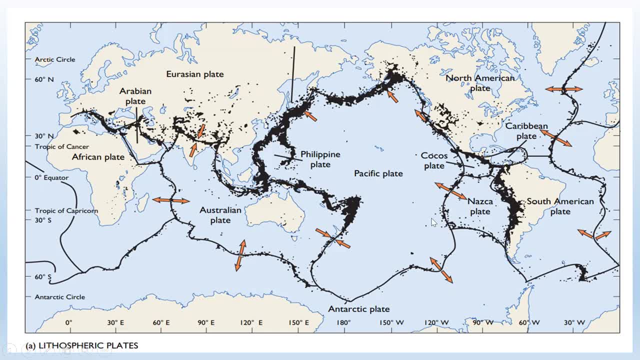 this in this image, the leap. now we are showing the movement of the basaltic plates and the reserching of the basaltic plates of different lithospheric plates. if you see the North Atlantic plate, North Atlantic plate- it is 20 centimeter. 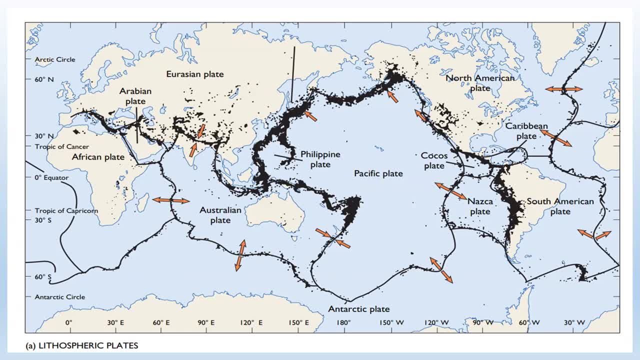 20 millimeter per year. it is the rate of separation of plate boundaries. here in the North Atlantic plate we are moving apart from each other, not Atlantic plate is moving apart from each other. so the rate is 20 millimeter per year. but if you see the 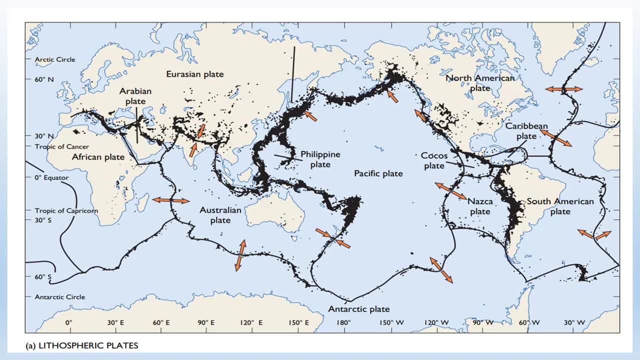 african and eurasian plates, the rates of closure: it is 10 millimeter per year and in the nazaka plate the rate of closure is 80 millimeter per year. nazaka plate is closing with the south american plate and and here the rates of closure is 80 millimeter per year. so if you see the 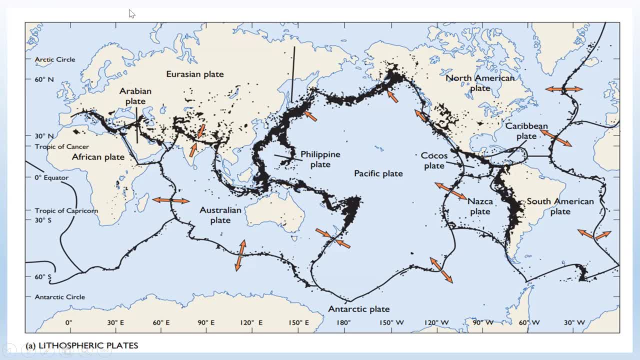 different rates. you can see that the plate motion is not constant. everywhere there is different rates of motions. also, this is very few, but the rates of motion is varying. it is not constant. so because now we will go to the next slide, where you can see the earthquake distribution zones along with different plate boundaries, here you see that the different 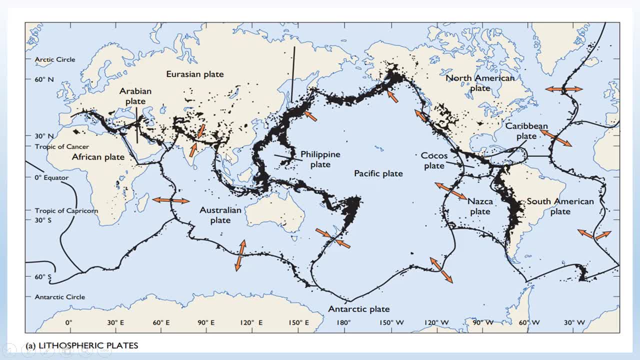 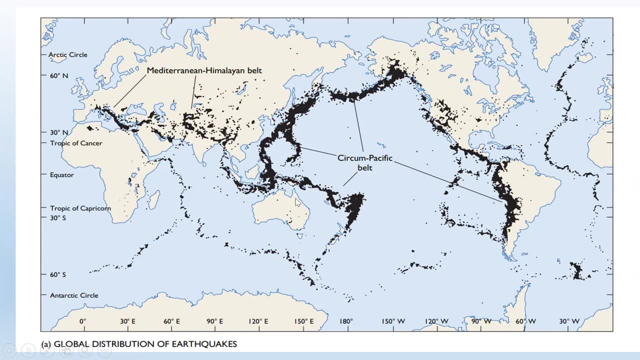 plate boundaries are the mostly earthquake prone zones. so which type of earthquakes? this, this map, is global distribution zone and this is the earthquake zone. so this is the earthquake zone of earthquakes, and you can see that the or the earthquake zones are nothing but the plate boundaries. these are, uh, these are correlated or these are. these are the zones of plate boundaries. 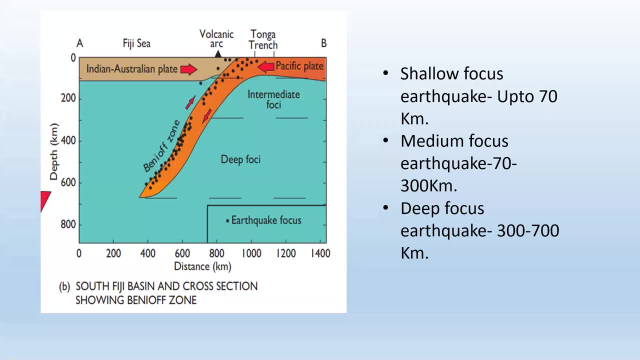 where disturbances occurs. now, if you see in that why these types of earthquake zones and five different earthquake zones is happening in different parts, these diagrams will show you something. some earthquakes we can show, say, as hello focus earthquakes, that is, they are up to the range of 70 kilometer. some earthquakes are medium focus earthquake, that 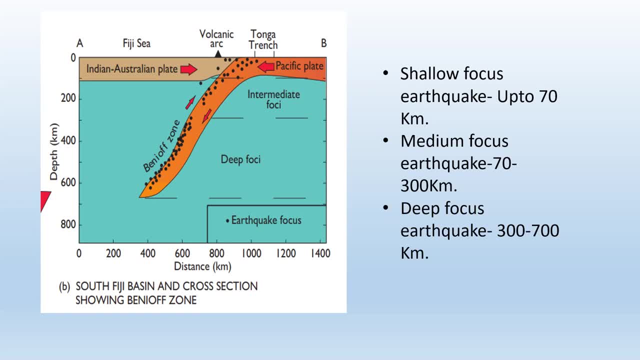 is they are they. they range up to 70 to 300 kilometer and the deep focus earthquakes ranges from 300 to 700 kilometers. now, you can see that this is a subduction zone model and this is the venue of zone. venue of zone, that is, the earthquake venue zones. venue of zones where different. 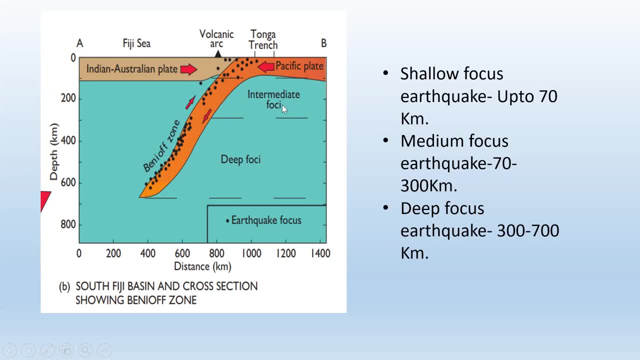 earthquakes are happening and uh, so the earthquake zones are not the same as the plate boundaries and intermediate focus earthquake, deep focus earthquake, shallow focus earthquake: all these things are are happen. all these things can happen in the subduction zone. all the major earthquakes are happening in the subduction zones, although, 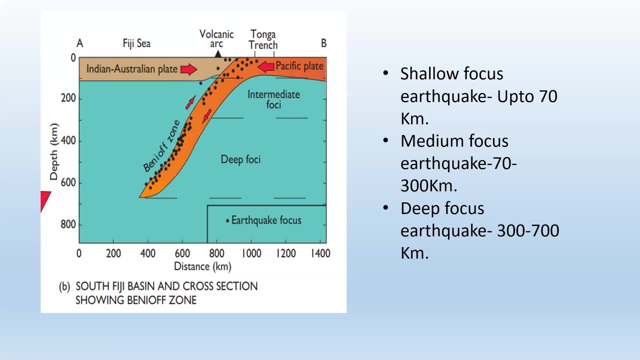 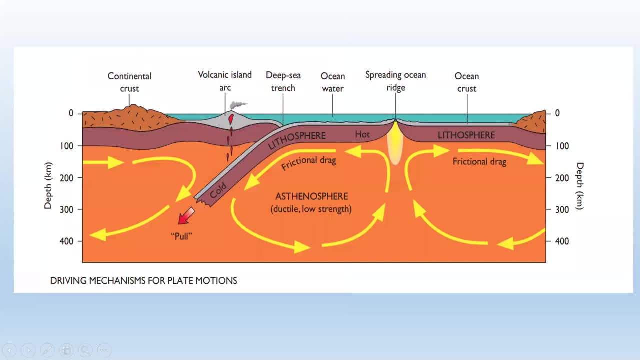 mediotionic region transform. pulse plate disturbance occurs there, but most of the very deep focus earthquakes happening in the subduction zone. now, if you see this model here, you can see everything together. that is the mediotionic reach, that is the subduction zone and here is the formation of trench. everything is there in this diagram. 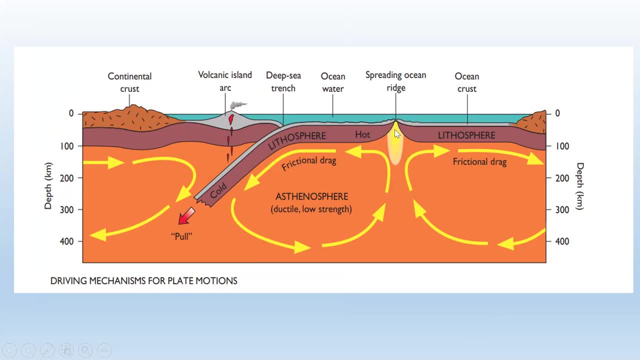 in the spreading range. in the spreading and spreading range, that is, in the mediotionic reach, very shallow focus earthquakes are happening. but in the subduction zones, deep focus earthquake happens, spreading in the spreading range, the plate in the spreading reach heat flow is highest at the ocean reaches because here the molten magma is coming directly to the 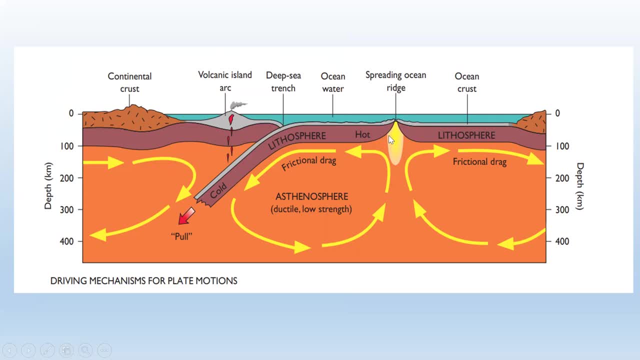 ocean surface through the mediotionic reach. so if you see the oce, if you think about the ocean basalt, a positive, positive magnetic gravity anomaly is there because of high density basaltic material. But if you come to the mid oceanic ridge, because of that molten magma, there is a low density. 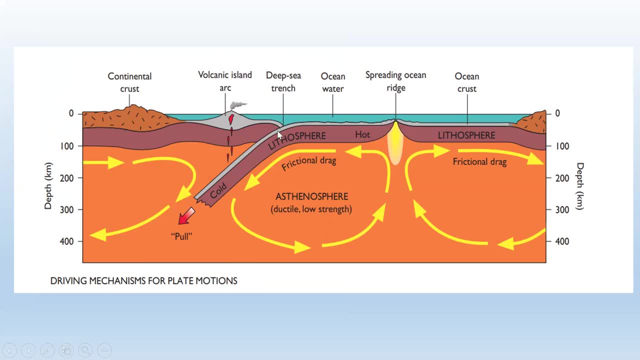 creates and there is a negative anomaly, is superposed along the overall positive anomaly, along the mid oceanic ridge, because here separation occurs. because of that, because of that high temperature, magma, high temperature and low density molten material at shallow depth in the crest and if you see, at the destructive plate boundary, here the ocean plates takes. 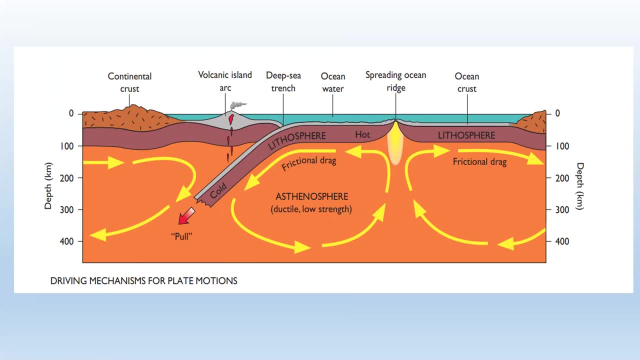 its oldest age- that is the maximum age- happens and this is the. this becomes the very cold and because of this they are the danger. and in the trench there are low density sediments, along with some water, muds, and all those things happens there and because of these along the 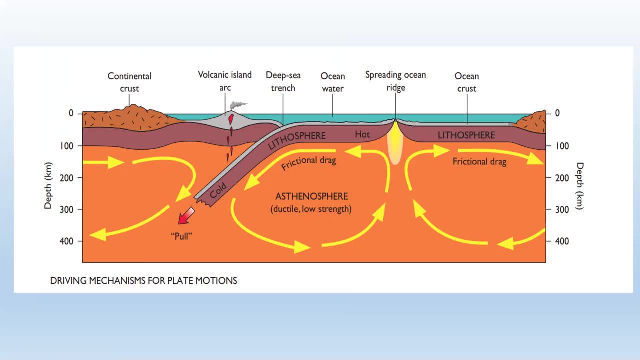 trench can find a very negative, negative gravity anomaly. but if you come towards the subduction Jones, towards the, towards the subducting plate down, you can see that in these positions the high density, many materials, that is equal guides and all those things forms. so because 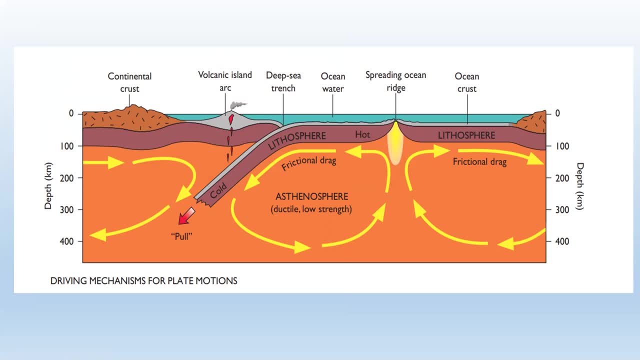 of these, the, because of these there is a positive gravity anomaly we can observe. so these are the gravity anomaly, ranges of constructive and destructive mount boundaries. I can say, and in these diagrams also you can say: see that the four are busy in back of busy in a Christian. 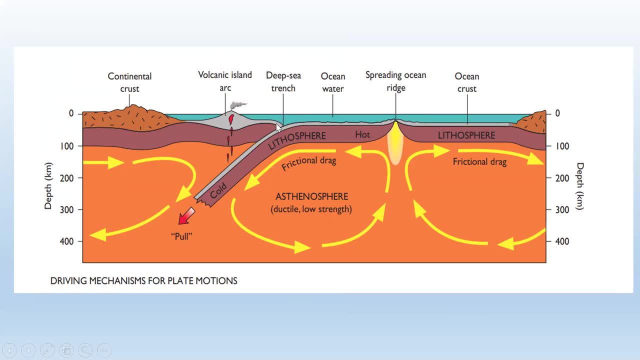 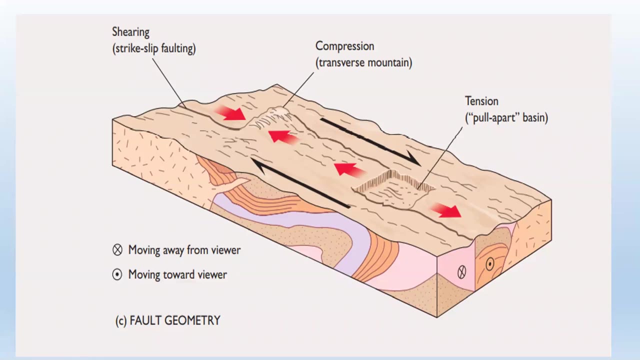 or Ephesians. these are the positions where a Christian or Ephesians developed. so these are Christian or Ephesians, are very important for exploration applications and all those things. now we will go to the next slide. that is, the structure of those ocean basins when there is a, when there is compression, because of this compression, 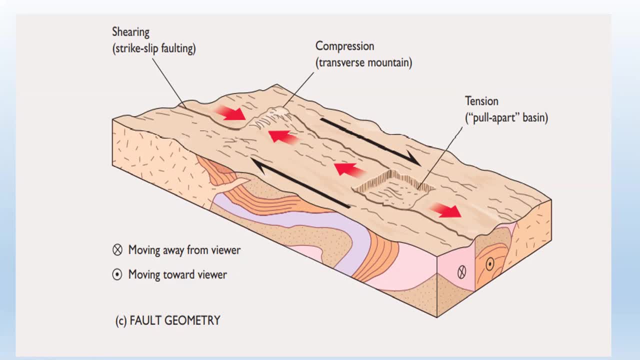 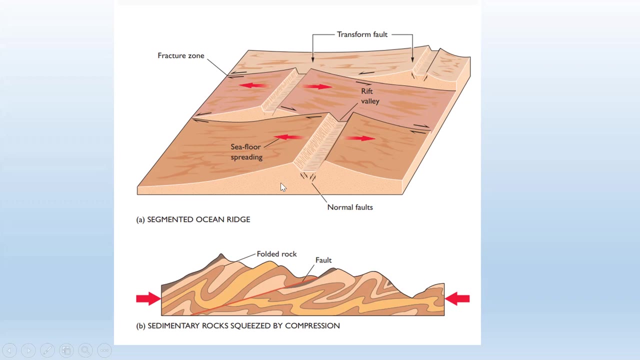 positive flower structures forms and, because of the tension, pull apart basin develops and negative flower structures forms. in this pool apart basins and in this compressive areas positive flower structures forms. if you see the segmented old ocean reach, this is the position of a ocean reach. now you have to know that. which type of fault is where in that, in that mid oceanic reach? 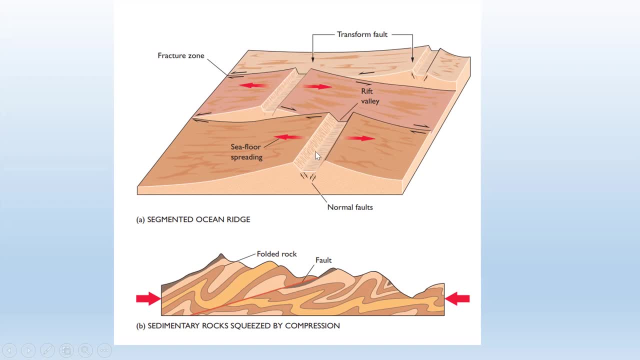 you can see the development of normal fault because here one plate is moving apart from another, that because of the tension where the one plate is moving apart from another, the, the plate materials sank and because of that normal fault developed along the mid ocean increase, but where the barbara 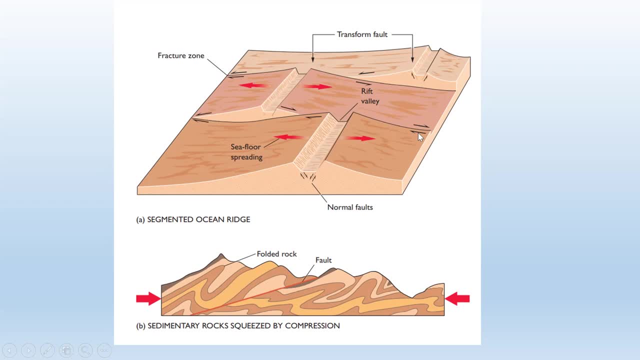 here you can see the transform faults develops during the breaking of that reef valleys, the transform part. in this diagram you can see that this is the position of transform faults. so throughout the ocean you cannot found the transform faults. transform faults are found in the ocean basins but in some places. you should know that, where the normal faults are developed. 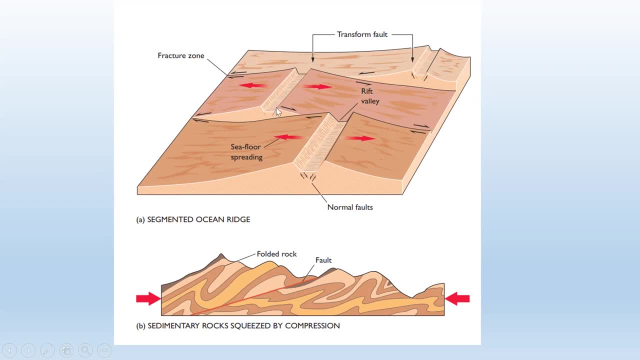 where they will be. these normal faults also are very few in amount or very bunches, but very precise with respect to the transform faults. transform falls are very fast. you can see that these are the all those thick, all those things forms and because of this compression, some